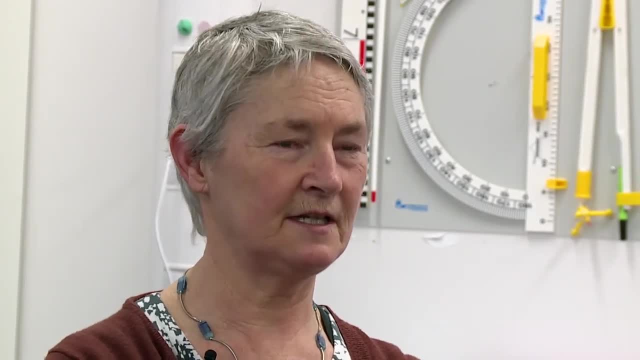 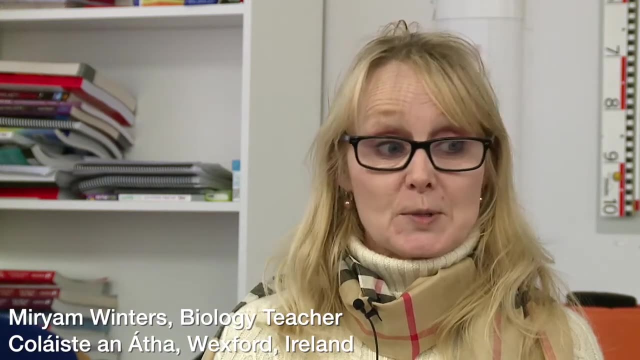 it once or twice, you would anticipate where this discussion is going. What we did here this evening, the finishing off, was absolutely fabulous. It was a little bit nerve-wracking. It was nerve-wracking at points when you were given the catch box, because you normally freeze. 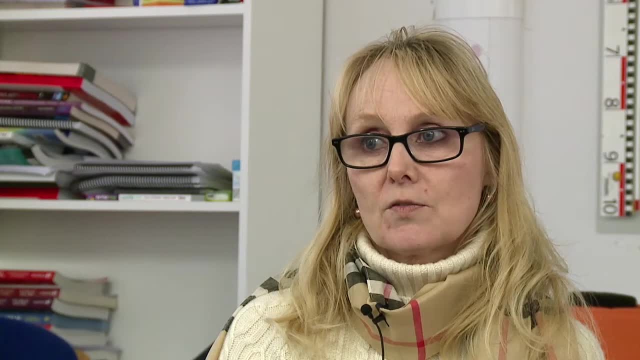 But we learned so much information on how we can apply that in our class: different classroom settings, not only in science but in other subjects. It's not something we're used to doing, is it, as science teachers is having these kind? 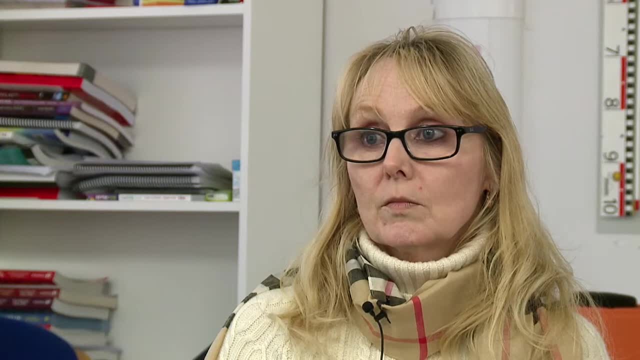 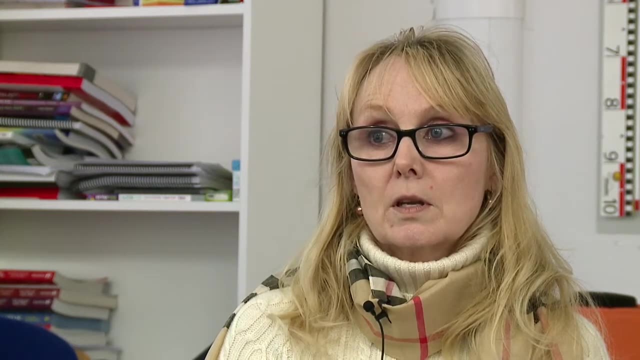 of debates that would. I suppose they'd be much more common in English classroom or the SPHE classroom or even the history classroom. I think, Yes, Not something that science teachers often get into, not in any kind of structured way. No, because we normally just deliver facts. 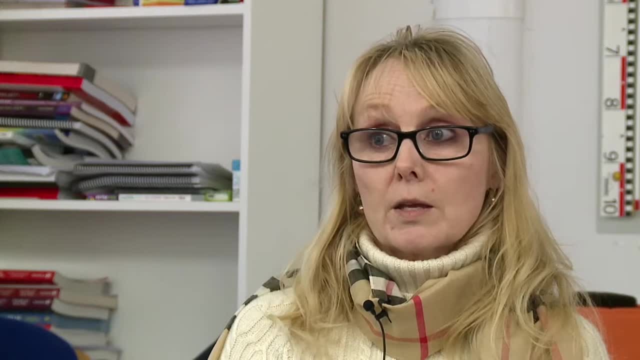 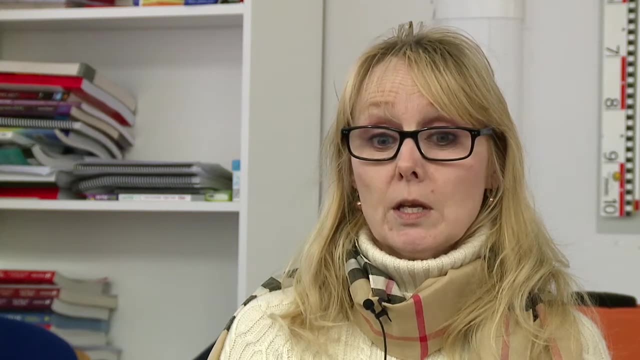 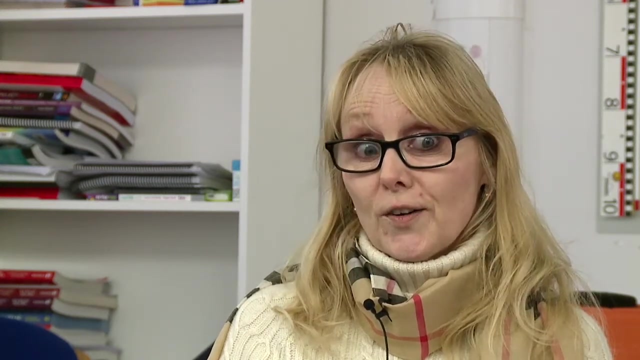 Yes, When it comes to ethical issues, this kind of set up for students is absolutely fabulous because it really engages everybody. first start, and it gets them thinking and no question is silly, or And they all get a chance to talk. And once there's ground rules set out, 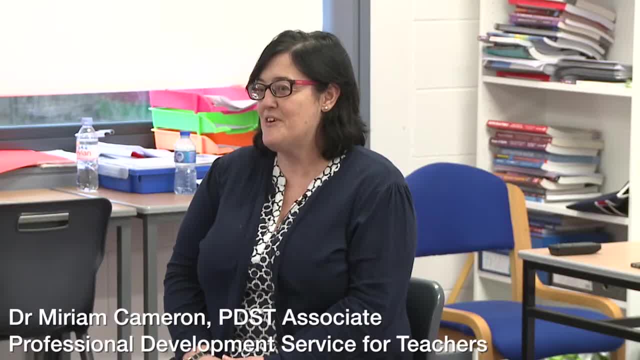 and they listen to each other and it motivates them to think. Kids will have heard things about CRISPR, but they don't know what to think. Kids will have heard things about CRISPR, but they don't know what to think. 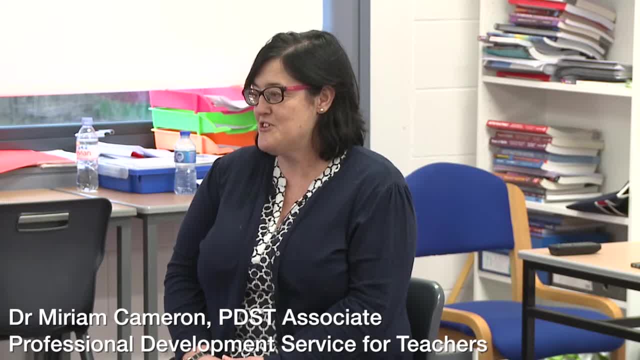 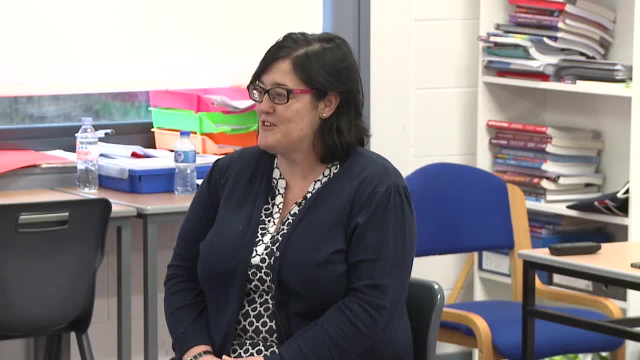 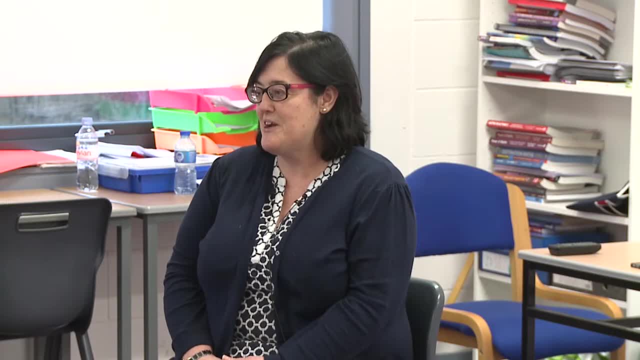 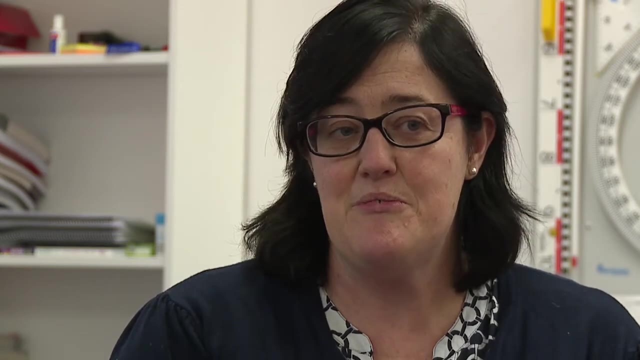 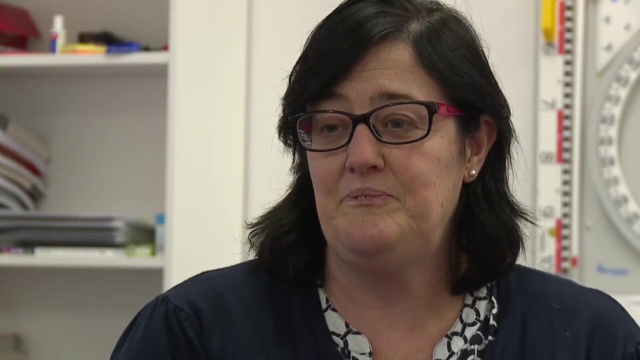 ethical issues and evaluating those issues around biology and around genetic information and genetic engineering. it's a great way to address misconceptions students can have, but allows students to develop real thinking skills, informed thinking skills, to be able to research and to be able to judge and make an opinion based on those. do you think that the philosophy activity 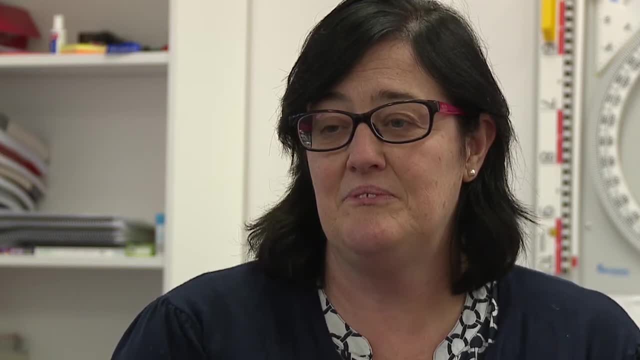 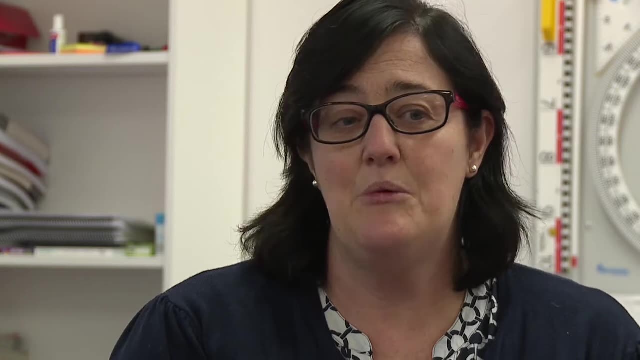 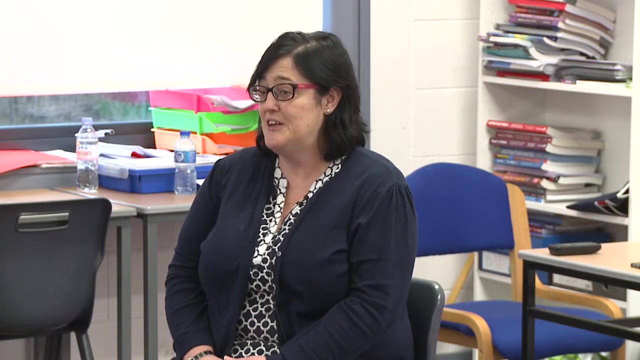 is potentially useful to biology teachers. you mentioned the key skills linking to this key skills and linking to this area. well, I think for the junior search, students have to have informed opinions on various subjects like sustainability, global warming, etc. but we're not really teaching children unless we teach them how to